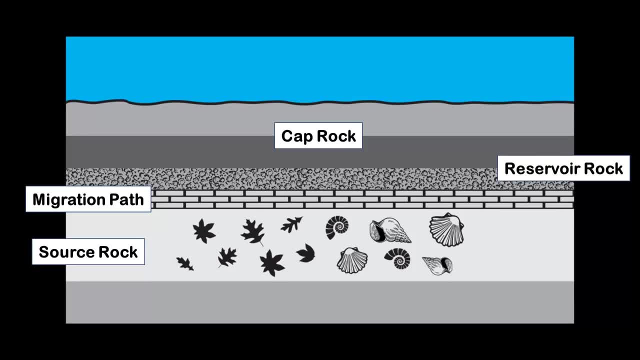 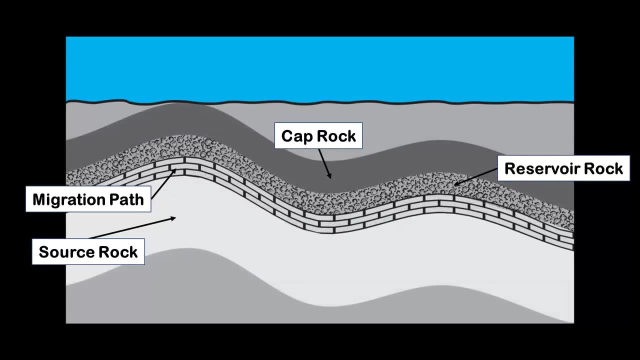 However, this flat cross-section is unlikely, as the Earth compresses and folds over time, producing in this case two anticlinal structures which reveal the last features for hydrocarbons- to be found, a trap or trapping mechanism. With these features intact, we will be able to use geophysical techniques to identify each feature and build a story which will aid us in exploring for hydrocarbons. 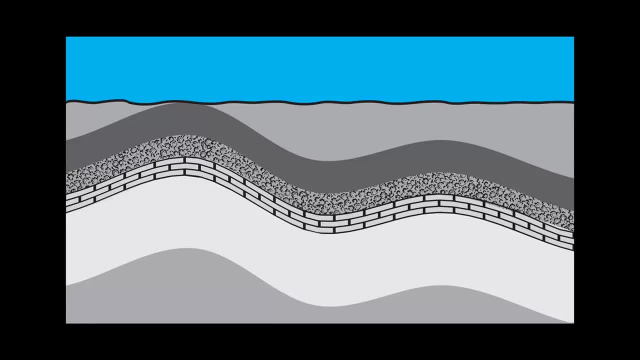 The story will include the following: The story will include the source rock which should be deposited at the proper time and be at proper depth for hydrocarbons to be created, A migration path- in this case, a permeable or former permeable rock- or path for the hydrocarbons to migrate. 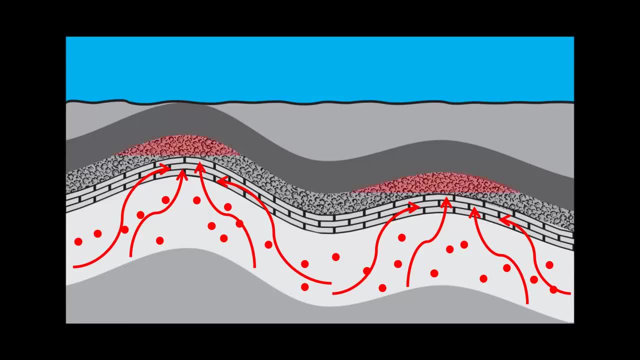 We want to tell a story about the reservoir rock, which needs to be porous to store hydrocarbons in mass quantities. We also want to make sure that the cap rock is impermeable and unbroken to stop the hydrocarbons from migrating out of the trap. 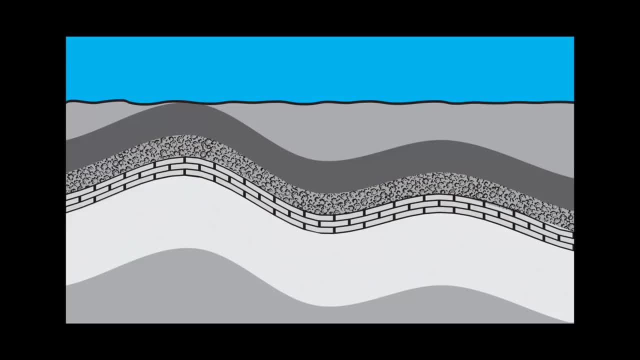 There are also some other features of these characteristics which we are also very interested in, such as the thickness of the source rock, to ensure that enough hydrocarbons have been created. the thickness of the reservoir rock to know how much hydrocarbons we can acquire. 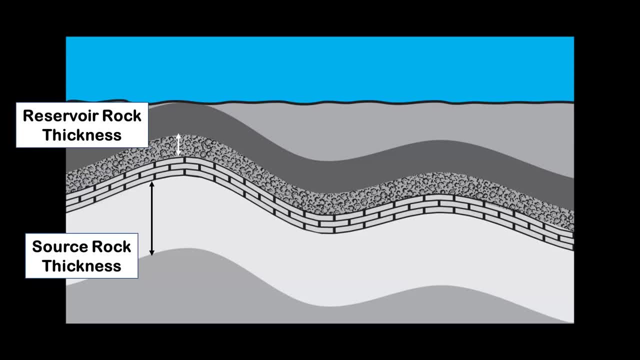 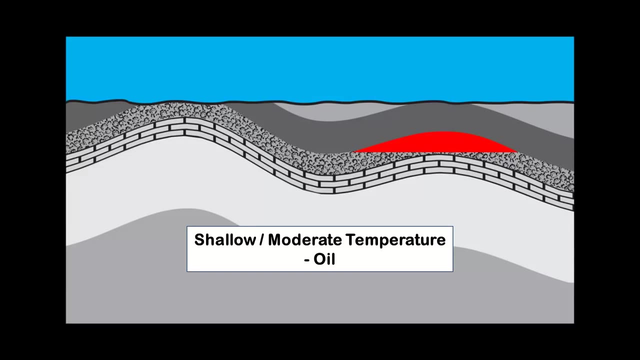 we want to know what type of organic material was present at the time of deposition: marine organics for oil and plant organics for gas. Further, hydrocarbon types are also based on depth and temperature. If the source rocks are shallow and cooked at moderate temperature, oil will be produced. 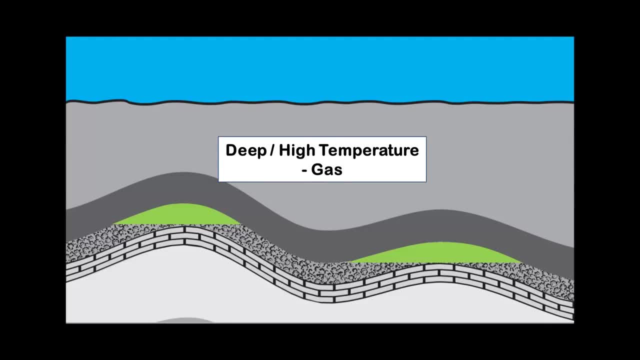 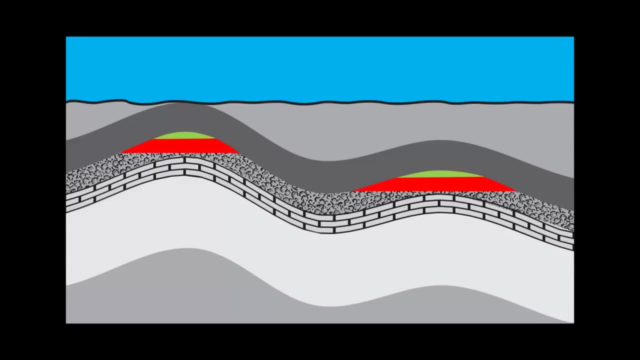 If the source rock is deep and at high temperature, gas should be produced, Or there is always the possibility that both oil and gas are present in the reservoirs. We also want to know the maximum extent of the trap, which is called the spill point. 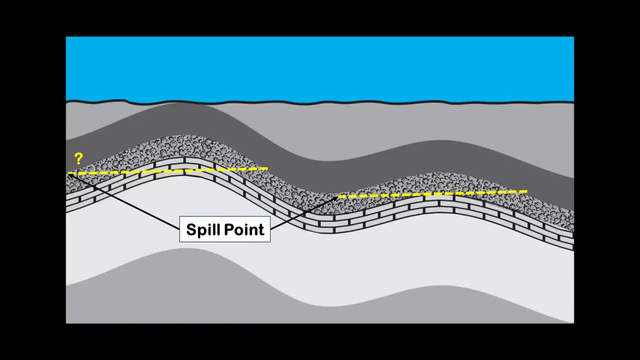 where the hydrocarbons will pour out of. We also want to know how much oil and gas are possible by looking at what is called the closure from the highest point in the trap to the spill point. The depth is important, so we know how deep we have to drill to find the hydrocarbons. 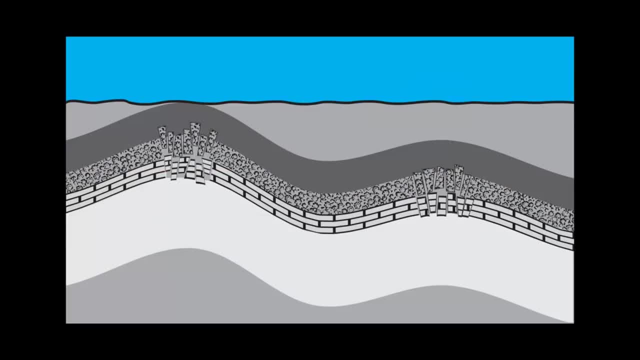 We also want to know about fractures. In this case, fracturing only affects the reservoir and migration path. Hydrocarbons can migrate from the source rock through the migration path and still accumulate under the impermeable cap rock. The increase in porosity of the reservoir from fracturing could even mean more hydrocarbons. 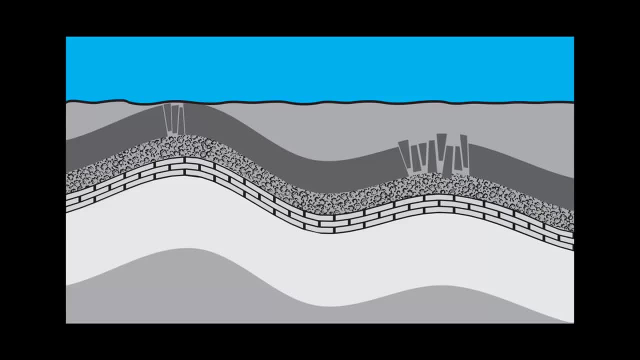 However, if fractures break up the cap rock, any hydrocarbons can easily escape, leaving the reservoir empty. In this case, the hydrocarbons move from the source rock to the migration path and continue through the fractured cap rock, leaving no accumulated hydrocarbons. 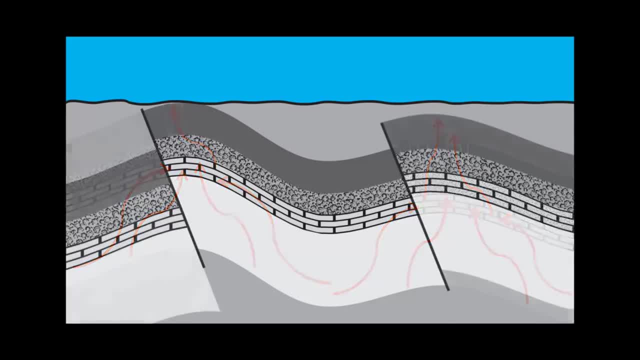 There could also be faulting within these structures. In this case, there are two faults: one advantageous for hydrocarbon accumulation and one which allows the hydrocarbons to escape. On the right, the faulting has moved the cap rock, but a seal still remains, allowing hydrocarbons to accumulate. 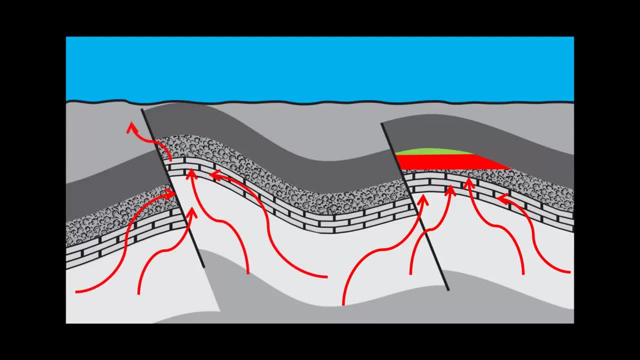 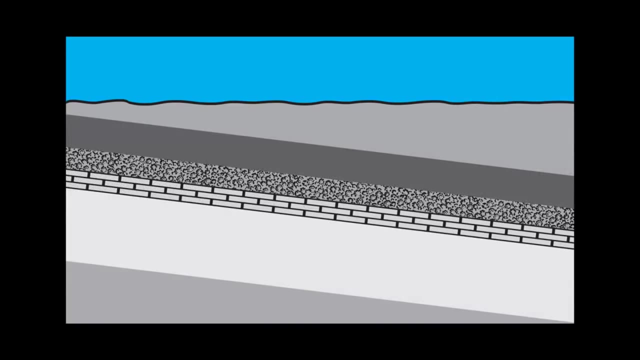 On the left, the seal is broken and the hydrocarbons can escape, with no hydrocarbon accumulation. This faulting brings up an important concept of timing of the geological structures. This laying was originally laid on the ground, but if the layers tilt, the petroleum still has a source rock, a reservoir rock and a cap rock. 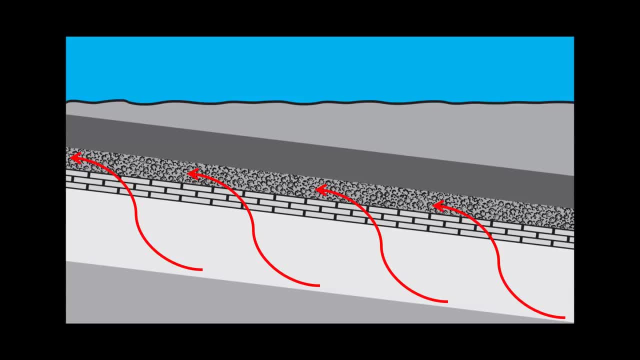 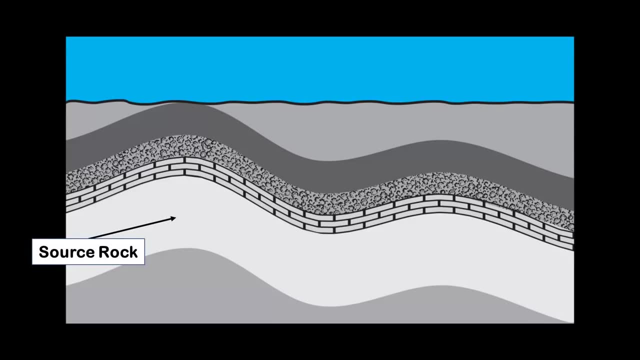 but the tilted migration path allows the hydrocarbons to flow up and away. Even after folding. we still have a source rock, an alleged migration path, a reservoir and cap rock and an anticlinal trapping mechanism. However, during the previous tilting process, 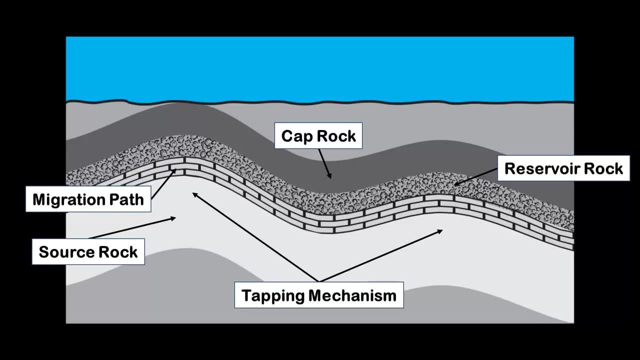 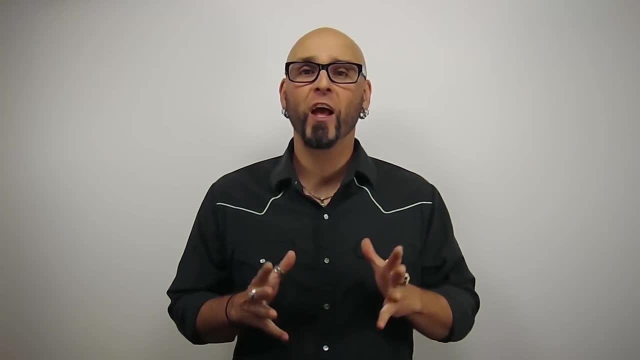 all hydrocarbons have migrated away, leaving the reservoir filled with water or nothing at all. This shows the importance that timing has for our features for hydrocarbon accumulation. To recap, there are five fundamental geological features that are required for hydrocarbons to be found. 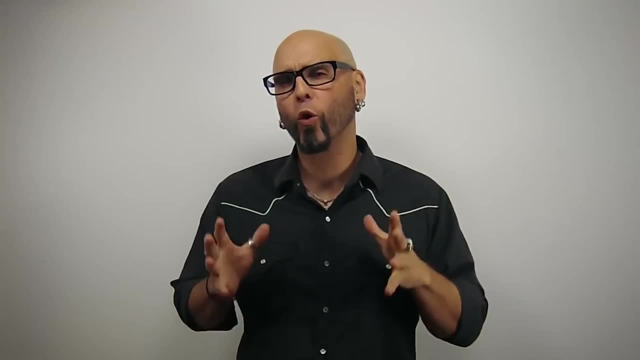 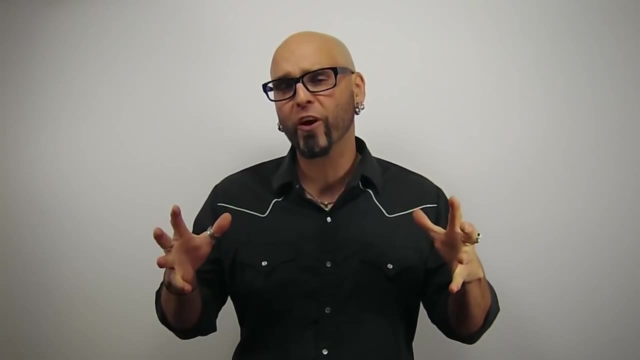 These features include: a source rock where organic material and sedimentary basins are buried and cooked over time into hydrocarbons. A reservoir rock which is porous enough to store hydrocarbons. a migration path for the hydrocarbons to move from the source rock to the reservoir rock.